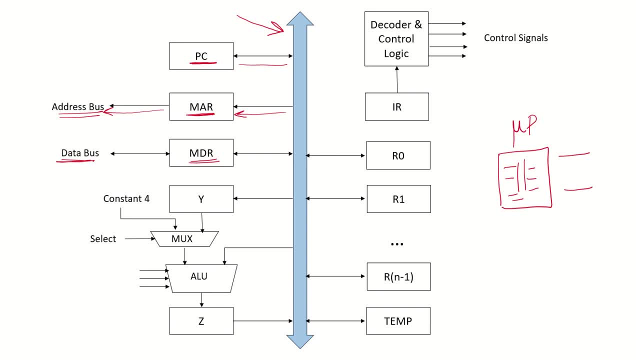 to the internal bus as well as the external data bus. We can see that this MDR has two inputs and two outputs, So one input is from the external data bus and one input is from this internal data bus. Again, the outputs are two: It can send to the data bus and it can also send. 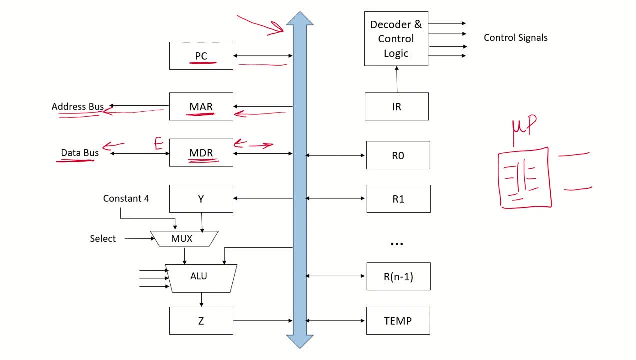 back to the internal data bus. So this is the MDR, So this is the MDR, So this is the MDR. So the MDR will send us the data from the internal bus. We have an ALU, We have these register. 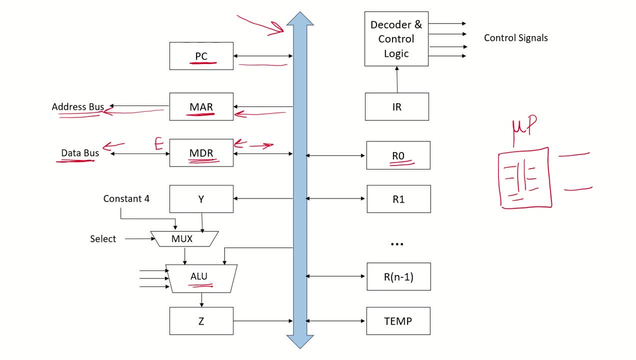 general purpose registers. So if there are N registers- so starting from R0 to RN, minus one, these are the general purpose registers which are also connected to the internal bus- Then we have an instruction register which will take input from this internal bus and 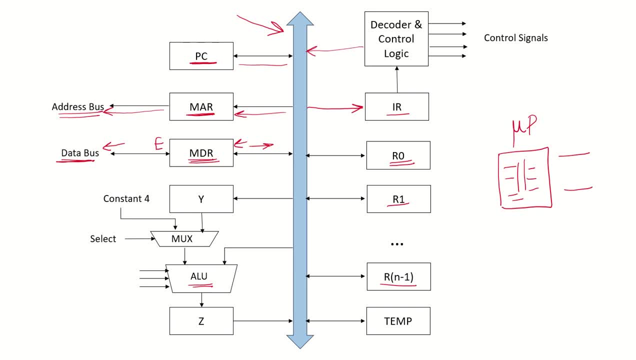 pass it on to the decoder and control logic, which can then send signals- control signals. IR is supposed to keep the instruction which is currently being executed and, once this instruction has been received in the IR, it is sent to the decoder and control logic, which will decode the instruction and generate appropriate control signals. 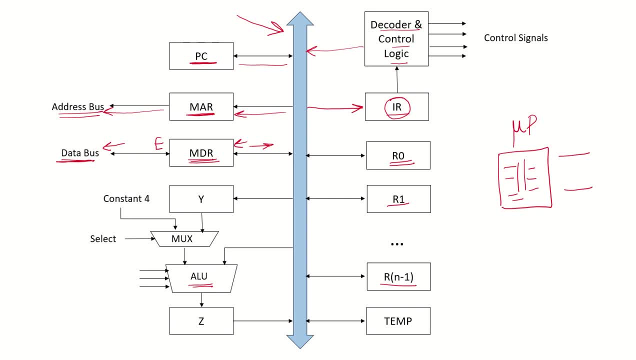 Now, apart from these, we also see there are certain temporary registers. They are Y, Z and Temp. This Y is connected to the input of a multiplexer and the other input of the multiplexer is connected to a constant 4.. The output of the multiplexer goes into one port of the ALU and the other port is getting 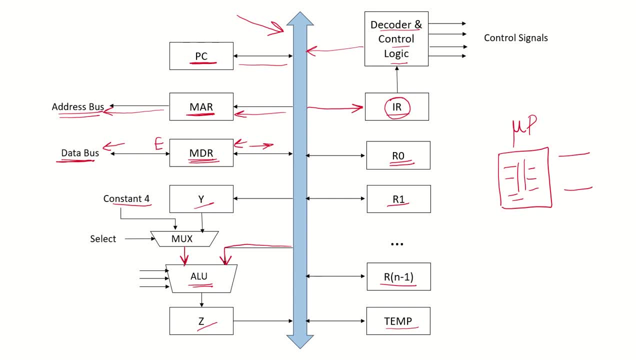 input from the internal bus, The computations that are done in the ALU, the result is put in the Z register and there is another temporary register which might be required By the processor for any temporary storage of data. So the constraint in this single bus organization is that at any given time, that means in any 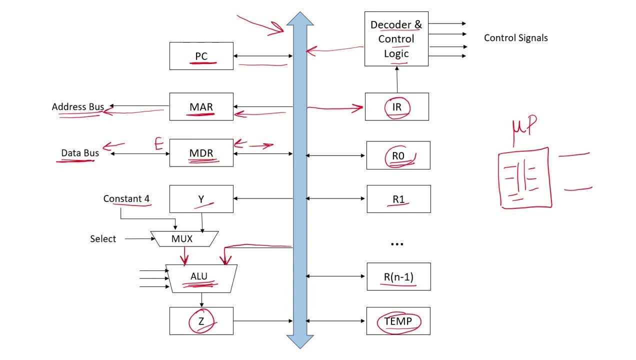 clock cycle, only one of these units can put the data on to the bus. So let's say, if MDR is putting the data on to the internal bus, so in that same clock cycle No other unit, No other unit Can put data on to the bus, though anyone can take data from the bus. 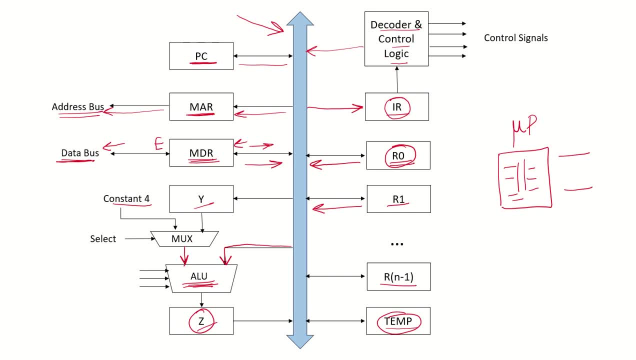 So in the same clock cycle only one unit can output on internal bus, but any number of devices can take data from that internal bus. So in any such organization where multiple units are connected to a bus, how do we control that which device Will take in data and which device will output data on to the internal bus? 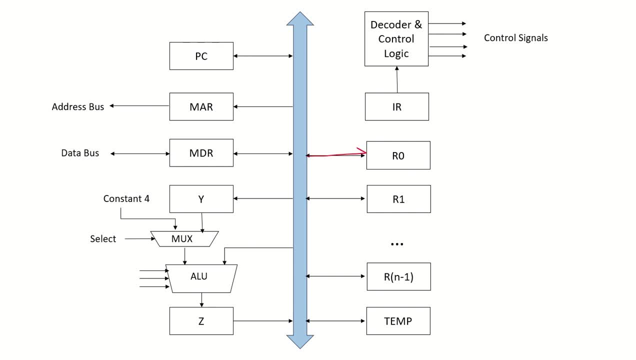 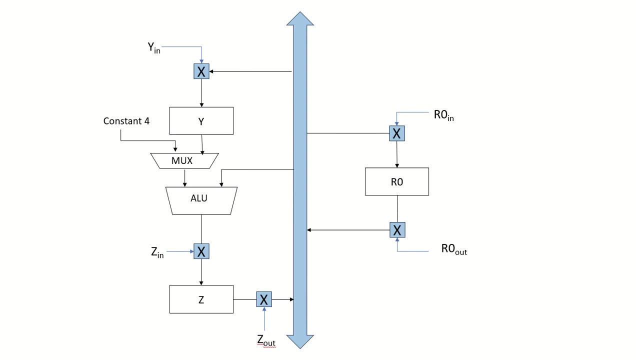 So right now we have shown like R0 as being connected to the bus in a bidirectional manner manner that means it can take data and can output data also. But actually there is a control signal associated with each of these units. So if this is the register R0, there is a control signal R0 in. 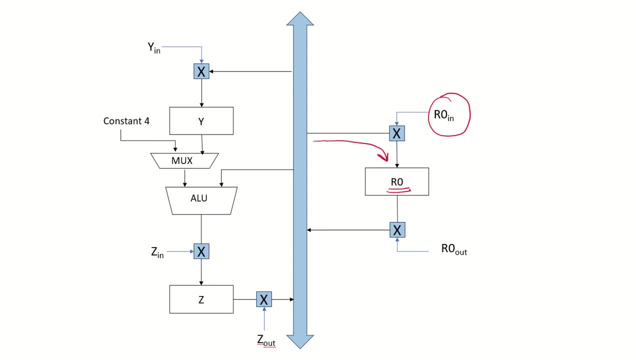 Which one Which will allow data to come from the bus into R0. if R0 in is not enabled, that means if it is 0, then even if data is here it cannot go into R0.. Similarly, if R0 wants to put data out on to the bus, R0 out has to be enabled and then only. 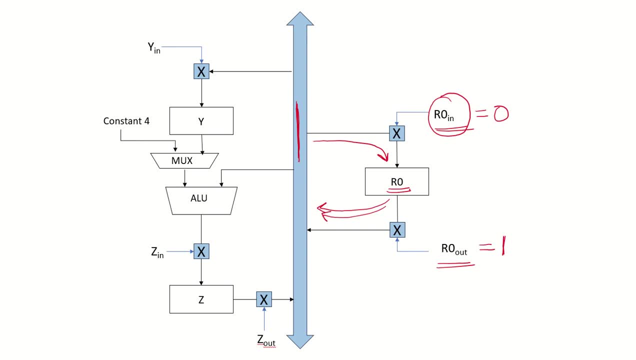 the contents of R0 can be sent to the bus. Similarly, Let's say there is register Y, the temporary register. it can be taking data from the bus only when this control signal Y in is enabled. Also, ALU can send the result of the computation in Z only if Z in is enabled and Z can output. 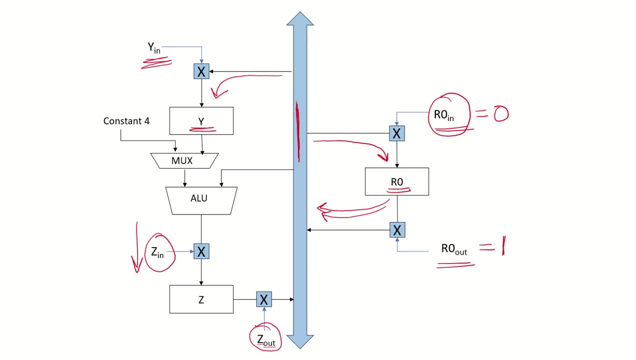 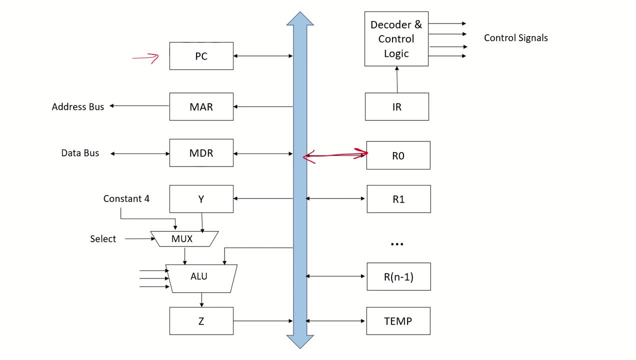 on to the internal bus only if Z out is enabled. So, similarly, each of these units that are connected To the bus, they have these appropriate control signals which will control their taking data from the bus or putting data out on to the bus. So why do we have this constant 4 as an input to the multiplexer? 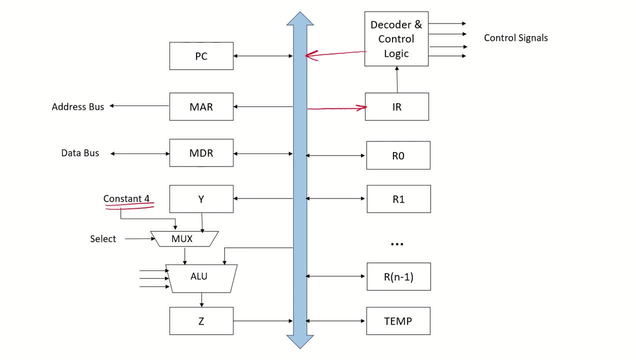 In this processor we are assuming, in this system, we are assuming that every instruction is of 4 bytes of length And the memory is biter length, And the memory is biter length And the memory is byte addressable. So if we have to increment the PC to point to the next instruction, PC has to be incremented. 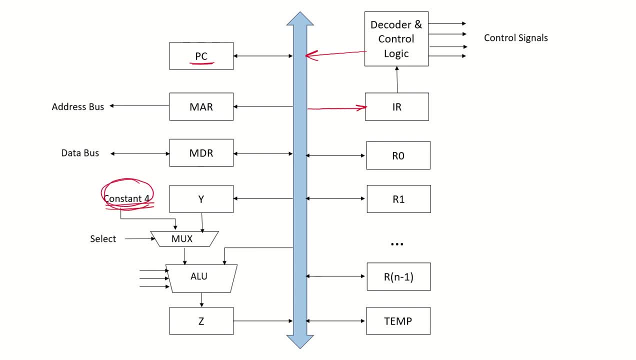 by 4, and so that constant 4 has been put over here. If the memory was word addressable, then the program counter would be updated by one address every time, and then we can put a constant of 1 in this case, so that PC can increment. 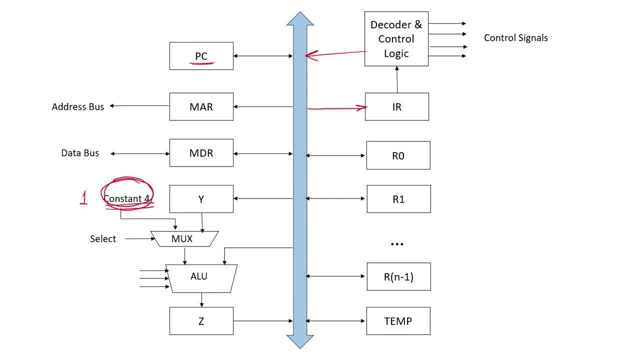 it to point to the next word. Now, this select will allow either this constant 4 to go pass through the ALU or, if it is a select Y, then this contents of Y will pass through the marks into the ALU. So, depending on this select signal, whether it is select 4 or select Y, the appropriate. 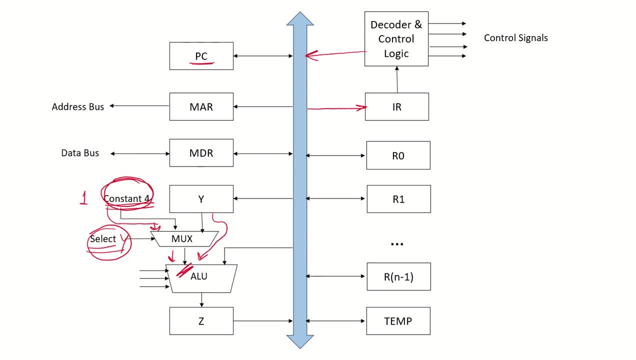 contents will be sent to this port of the ALU. Now, depending upon the number of operations that the ALU can perform, there will be a certain type of AMU which will be set. This is the type of AMU, which is the type of AMU, which is the type of AMU which is the 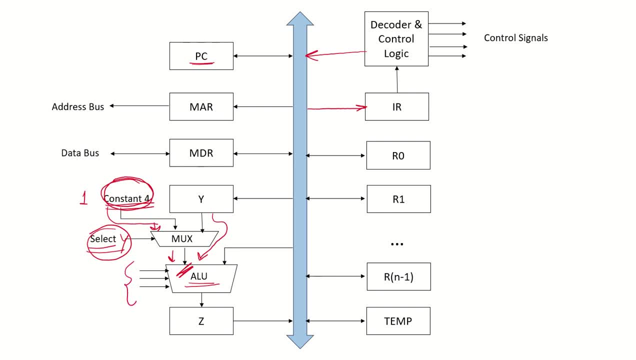 there will be these control signals that will be given to the ALU. Let's say the ALU can perform 16 operations like ADD OR NOT SUBTRACT, MULTIPLY. So these 16 operations can be controlled by either 16 control lines, one for each operation. 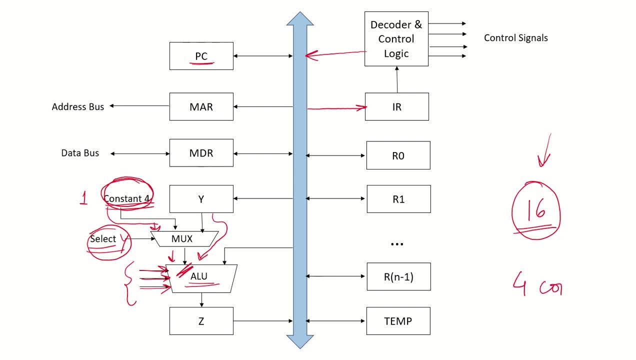 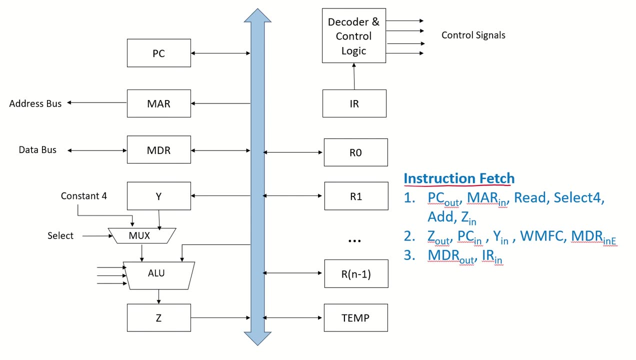 or we can encode this and have 4 control lines, and in that case each combination of these 4 control lines will specify one operation. Let's consider this instruction, FETCH. So we know that every instruction goes through the FETCH DECODE and EXECUTE cycle. 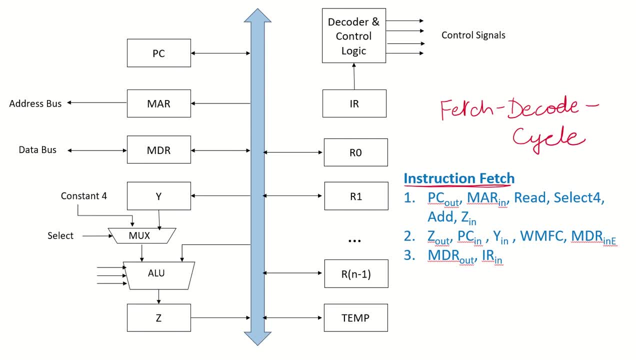 So let's see first how the FETCH will happen. So, since the instruction has to be FETCHED, the program counter has to send the address to the memory address register, because from memory address register the address will be sent out to the address bus. So for this to happen, what will be the sequence of the control signals? 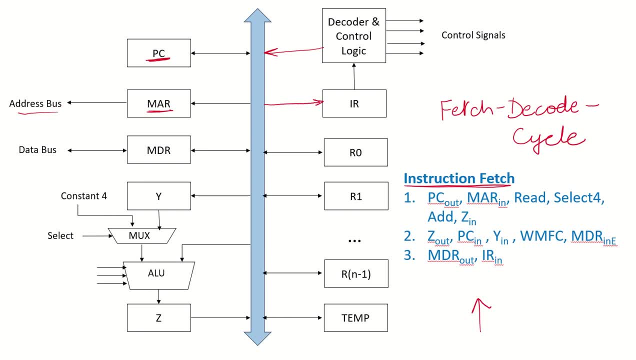 So this is the control sequence: PCOUT. that means the contents of the PC have to be put onto this bus For them to go to this MAR. So we will put enable this control signal, PCOUT. so the contents of PC now go onto the. 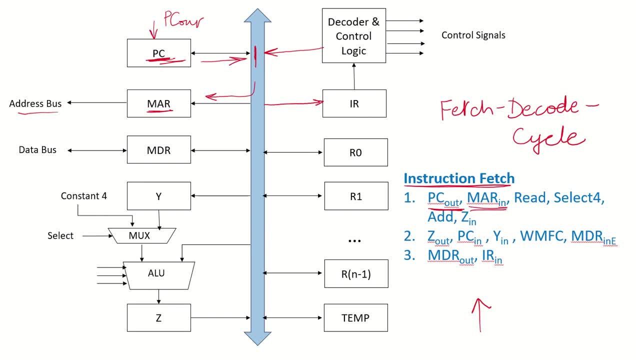 bus We have MARIN. so this control signal MARIN will allow the contents of the bus to go into MAR and we are assuming that as soon as MARIN is enabled, this external port is also enabled and the bus can have the contents. So we will put the contents over here and the address bus will take that address to. 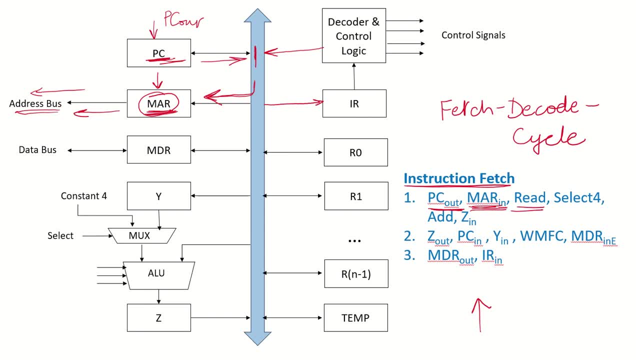 the memory. We will send a read control signal which tells the memory that it is a read operation. Now also, we want to increment the contents of PC. to point to the next instruction, These contents are already available on the bus because the program counter has put them. 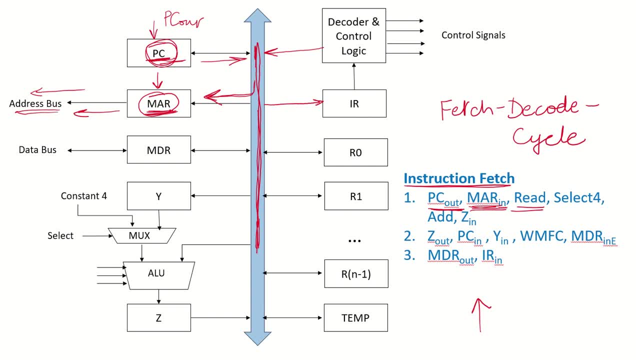 onto the bus. So We know that in the same clock cycle we can take these PC contents and we can send this constant 4 via the MUX into the ALU and do PC plus 4 and put the result in Z, So for that PC is already available on the bus. 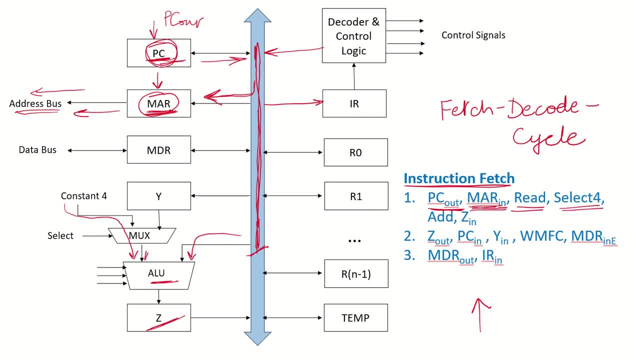 We do a SELECT 4 so that 4 can come onto this port over here We do an ADD operation And We enable the input of Z by doing a Z in control signal. Can we output on the same? can we output this PC plus 4 onto the bus in the same clock cycle? 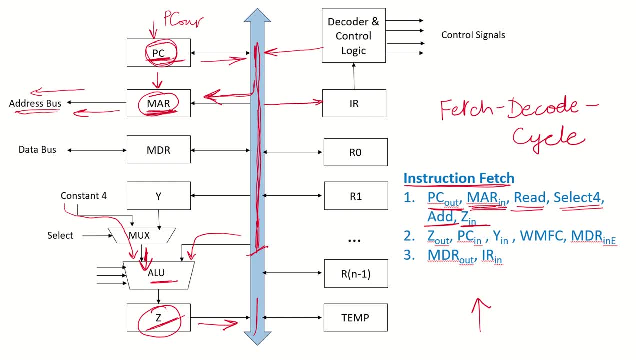 No, Because the constraint is that at any given clock cycle or any given time only one unit is allowed to put on the bus. and in this clock cycle PC out is already there, So the contents of program counter are already there. So in this clock cycle Z contents cannot go onto the bus. 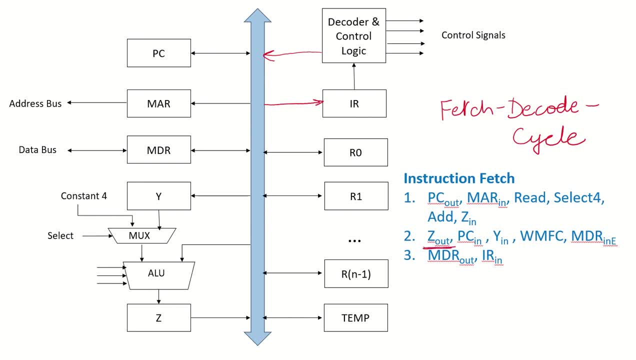 So in the next clock cycle we do a Z out. This is the control signal. So PC plus 4 was here. This will now be put onto the bus. It will be taken inside the program counter through this bus by enabling PC in. 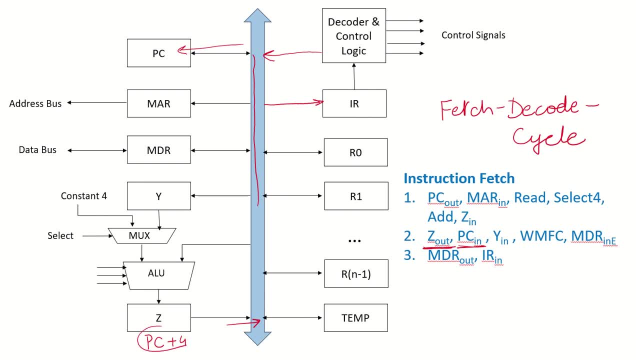 At the same time we also send this PC plus 4 into Y, one of the temporary registers. Why we are doing this I will explain later. So what we have done is that the updated contents- PC plus 4- we have sent to the program counter. 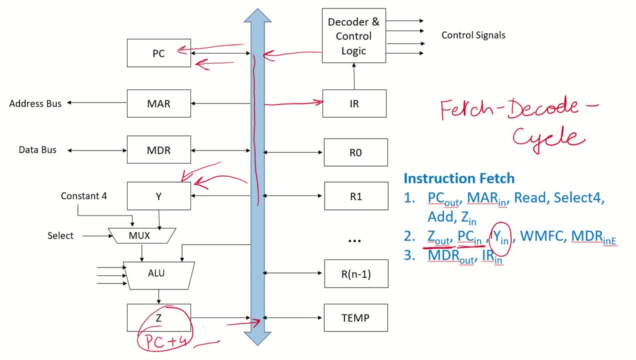 But at the same time We have also put in this temporary register Y. Then there is a signal which says WMFC, which is wait for memory function complete. So because this address has been sent to the memory, it is going to take at least one clock. 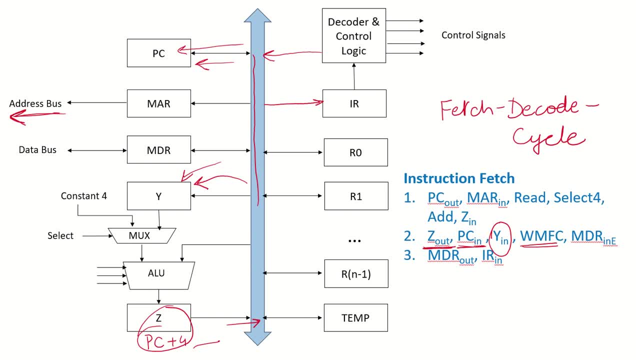 cycle to bring the instruction back. and when the memory completes its task it sends a memory function complete. So this signal- memory function complete- will be sent by the memory to the processor when the memory has finished its task. So we have to wait for that signal. 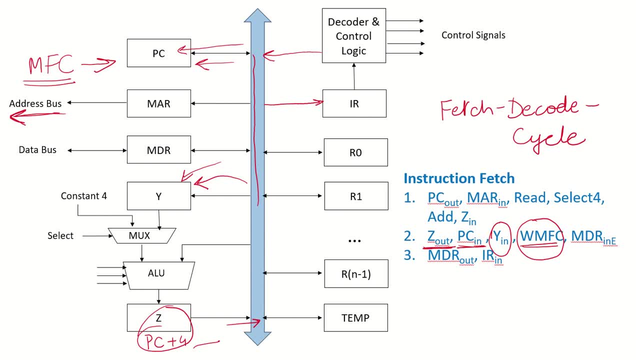 So we are waiting for that memory function, complete signal. It will take at least one clock cycle if that instruction is found in the cache. but if it is not found in the cache Then it is going to take more clock cycles if the main memory is accessed till the time. 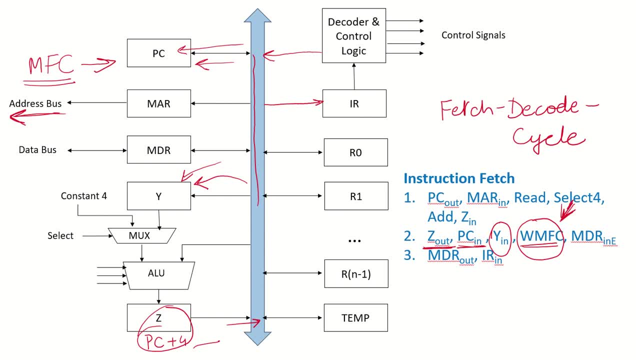 this signal is received from the memory, further instructions, further signals of further micro instructions will be put on hold. So the further actions will not happen till this instruction is received from the memory and the processor knows this because it has received a MFC memory function. complete signal. 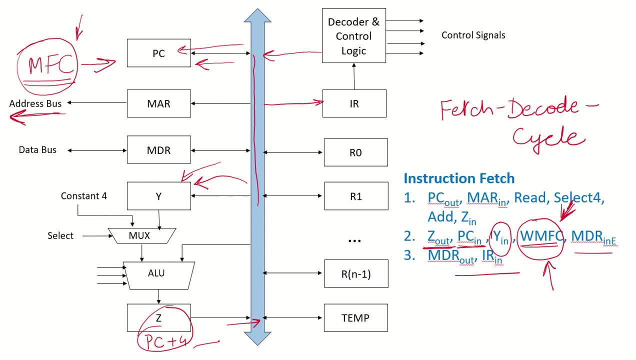 So we are waiting for that signal. If that signal is received, we have enabled the MDR in external. So this is the MDR in external, because this is the external bus and this is the internal bus. So we have enabled the external input. so the instruction has now come into MDR. 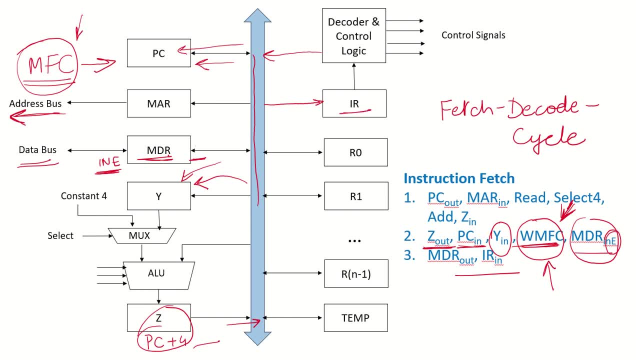 Now from MDR we have to send it to IR. But we cannot do it In the same clock cycle through the bus because in this cycle we have already done a Z out. So in the next clock cycle there will be an MDR out.